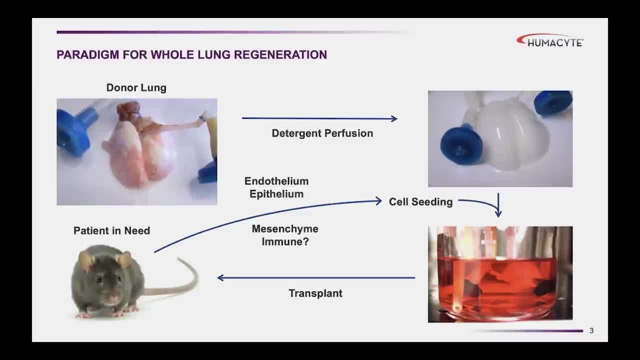 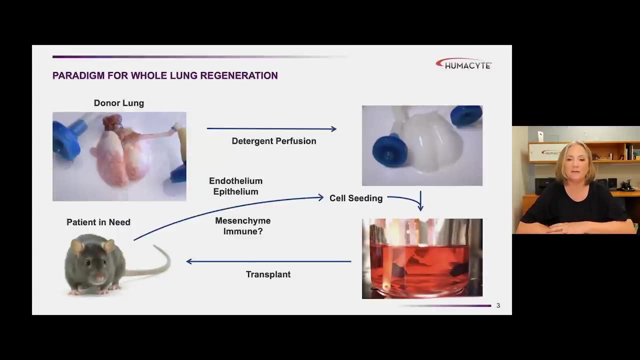 lung cells, such that we could reconstitute an organ that could actually participate in gas exchange for a few hours. This report came out in Science in 2010.. And, frankly, at the time when we showed that we could repopulate an organ and achieve gas exchange even for a short period. 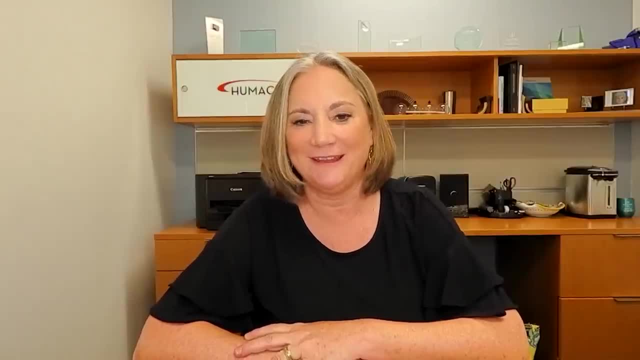 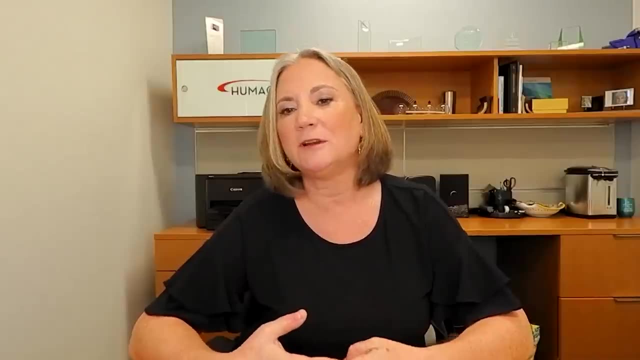 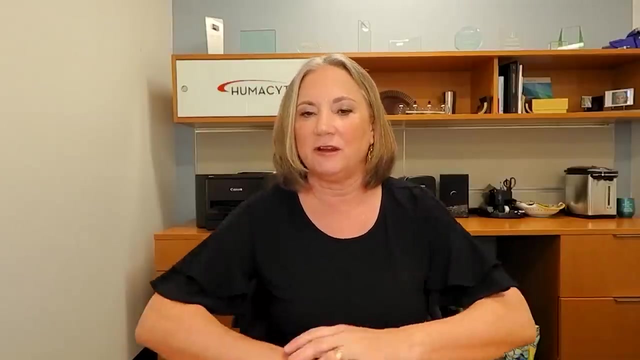 of time, I was actually flabbergasted that that was possible, But since that time we've really been working from these initial prototypes and really trying to hammer out some of the obstacles that stand between us and engineering a lung that can exchange gas in the long term. So, as I always say to my students and postdocs: I'm not going to go into too much detail on this, but I'm going to go into a little bit more detail on this. but I'm going to go into a little bit more detail on this. 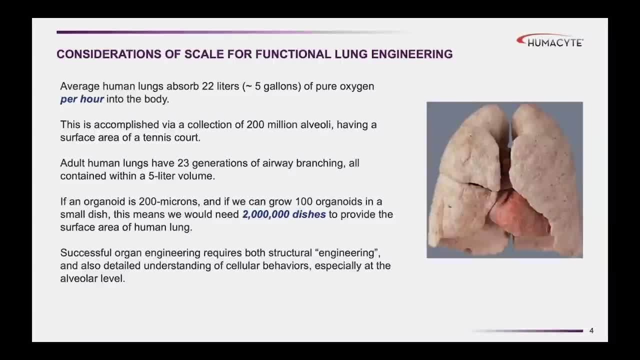 you know it's important when you're thinking about regenerating a tissue that you want to be functional, it's critical that you think about the key- what we would call design criteria- that go into whatever you're going to engineer that's going to really drive function. And there 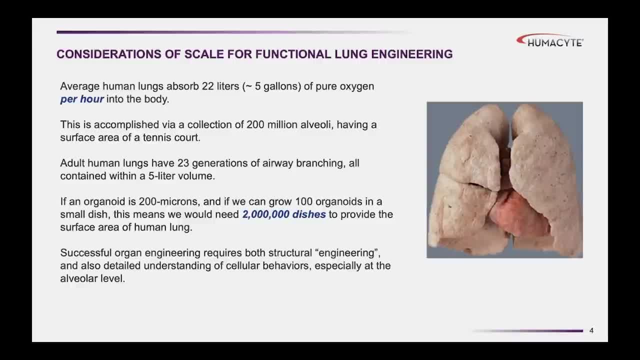 are some fun facts about the human lung. You know, the average human lung absorbs about five liters of pure oxygen every hour, which is actually a large volume of gas, And it also excretes a similar volume of carbon dioxide every hour. This is accomplished through 200 million alveoli, each of which is about 200 microns in diameter. 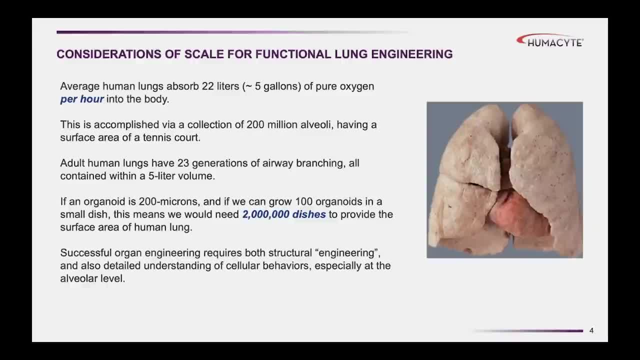 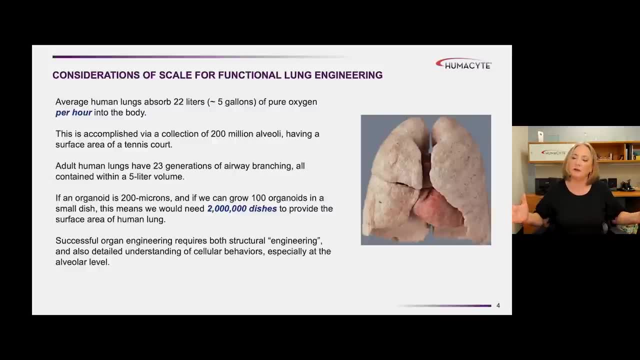 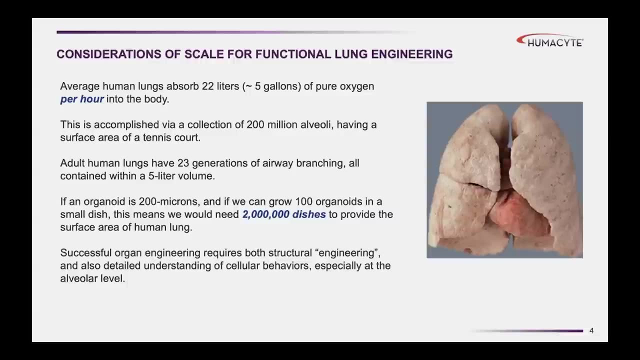 And with the 23 generations of airway branching, there's actually roughly 70 square meters of surface area in your chest which is useful for gas exchange and which provides this highly efficient gas exchange surface area. But if we think about what it would take to reconstitute a set of functional human lungs, one of my favorite facts that I tend to quote with stem cell biologists actually is that if we had organoids that we were growing in hydrogels and if each of those organoids was 200 microns in size, we would need roughly 2 million dishes to get enough organoids to reconstitute a full human lung. 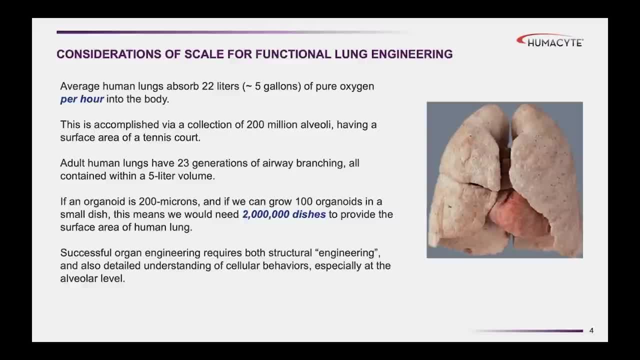 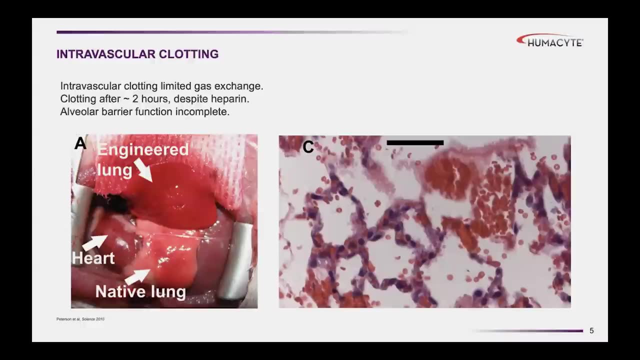 And so clearly just growing small little organoids that represent individual alveoli is not going to get us really to a functional organ. So as I mentioned we have in our early studies: we took acellular lung matrices that we carefully decellularized to really retain the alveolar structure and the microvascular structure. 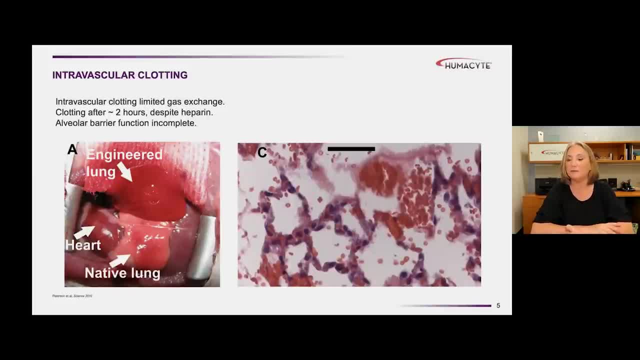 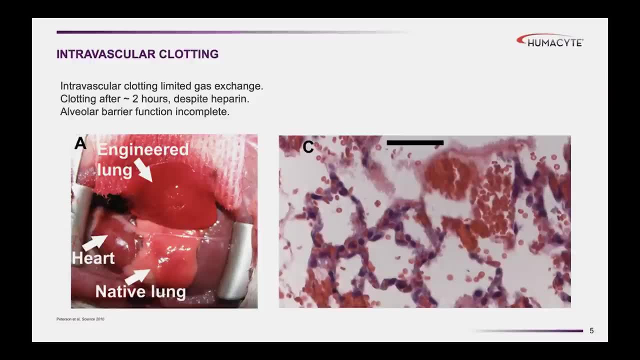 And when we repopulated these organs and then implanted them in vivo, what we found was that the primary failure mode actually was intravascular clotting. So you can see an engineered lung that had been implanted into a rat for several hours on the left and what you see is that it's sort of this beefy red appearance, and that's because there was a lot of microvascular and intravascular coagulation. 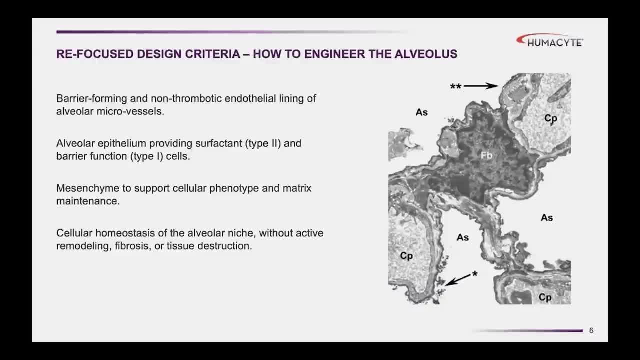 So this really led us to think very carefully about the alveolus, which is really the functional unit for gas exchange in the lung, And really the alveoli in your lung are replicated millions of times over And they're a fairly stereotypic structure. 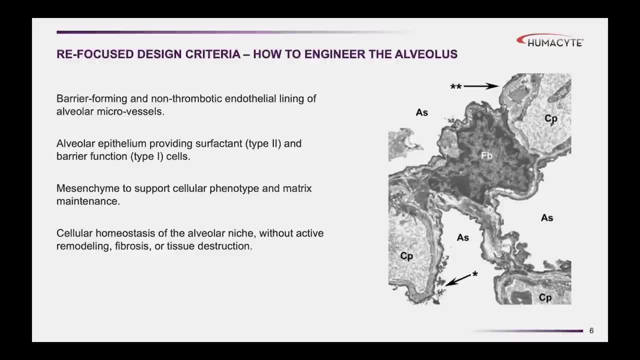 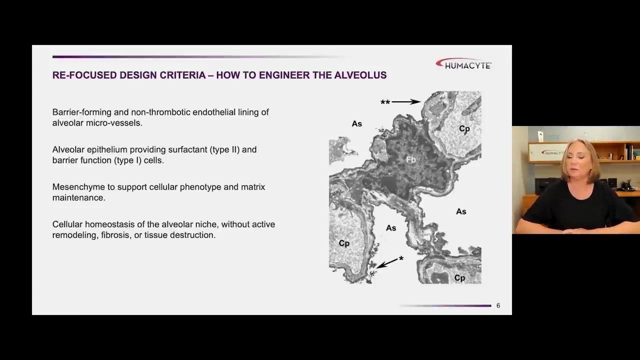 They contain about six or seven different cell types, including microvascular endothelium on the vascular side of the barrier, but also a collection of fibroblasts which sit in the septae, in the wall of the alveoli, And also they contain epithelial cells, actually of two flavors: type 1 and type 2 epithelial cells. 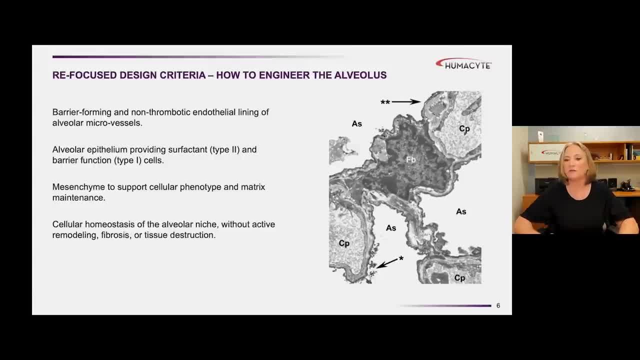 And the type 1 epithelial cells are the ones that are the most common. And the type 2 epithelial cells really stretch over the surface of the airway and sit right on the other side of the basement membrane, right next to endothelial cells. 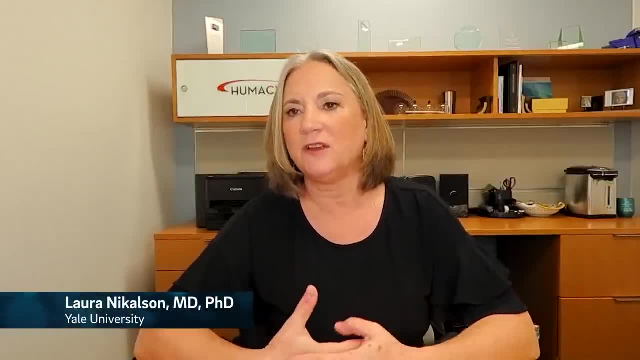 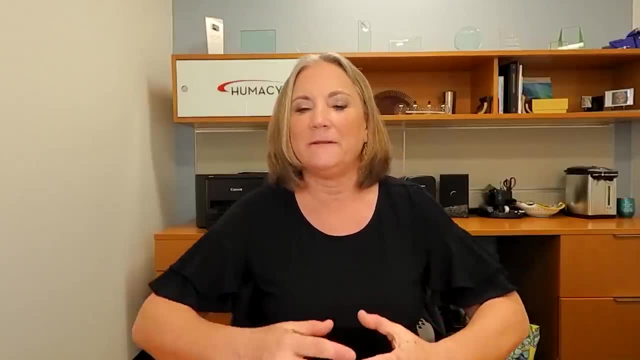 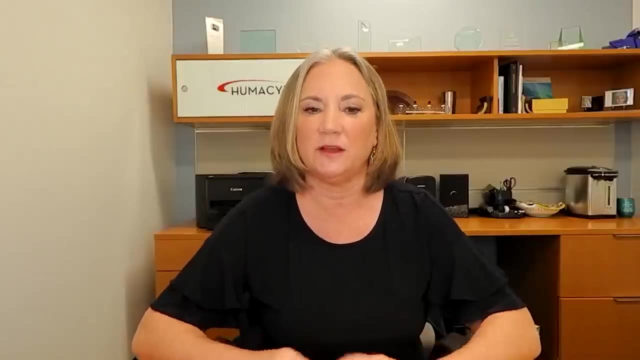 And I'll show you later on in this talk that we've done some single-cell analysis to try to understand how these neighborhoods or collections of cells talk to each other in the normal alveolus. But just to start, this just sort of orients you to the different types of cells that are located in the air sac. 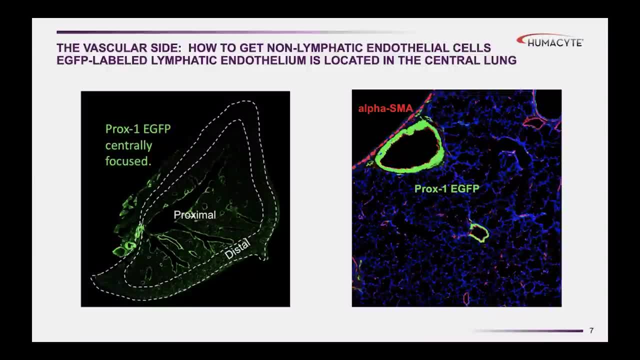 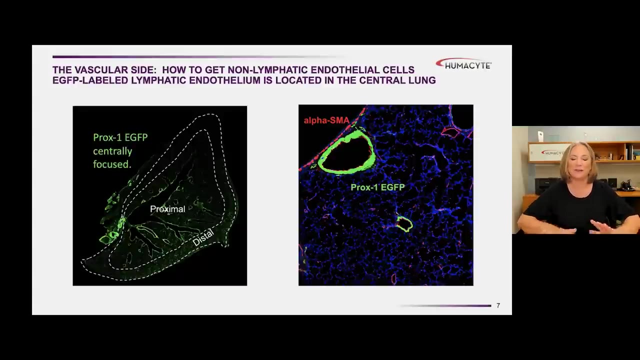 So when we began focusing more on providing a stable and complete endothelial layer in the vasculature in order to avoid clotting once we implant the lungs into native living animals, we realized at first that there's actually two flavors of endothelium: two broad flavors of microvascular endothelium in the lung. 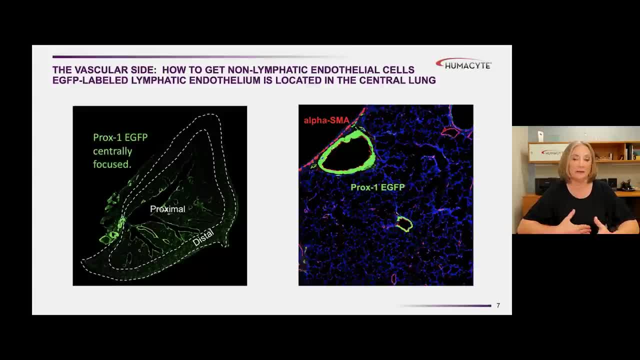 One is what we call blood endothelium, Which comes in contact with the blood stream, But another form of endothelium is lymphatic endothelium, which, as the name implies, lines all of the ducts of the lymphatic system. 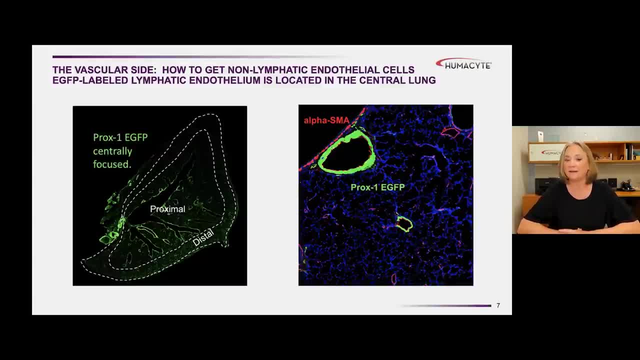 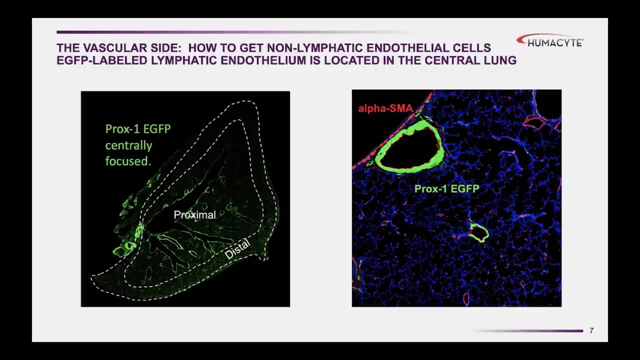 And there's actually a large lymphatic system in the lung that's very active. The endothelium of the lymphatic system is, by design, much leakier than the endothelium of the blood system, And so we became interested in really identifying the endothelium. 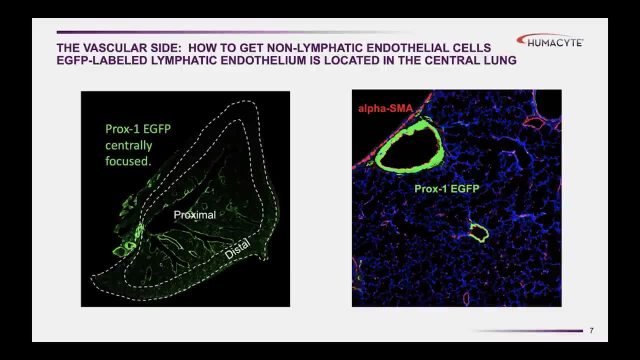 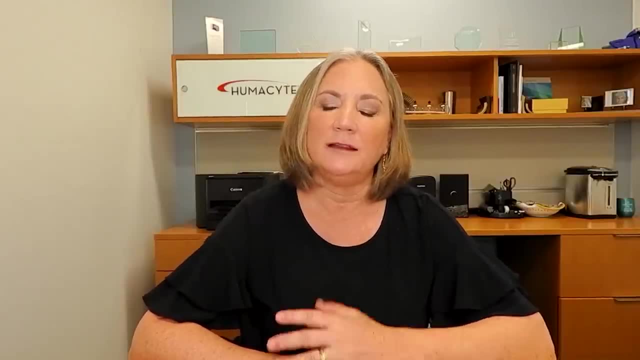 Endothelial cells of the lung. that would be blood endothelium as opposed to lymphatic endothelium, And blood and lymphatic endothelium share a lot of markers But there are some distinctions. So we obtained a transgenic rat that labels all of the lymphatic endothelial cells with EGFP. 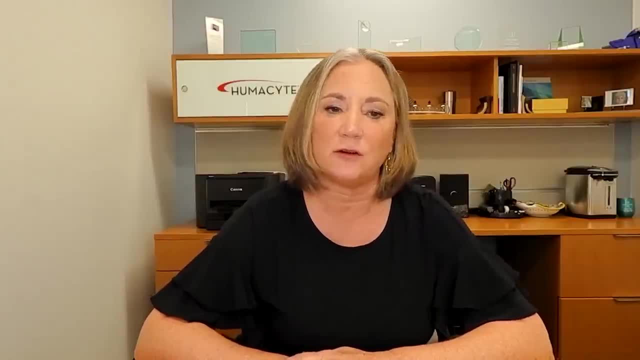 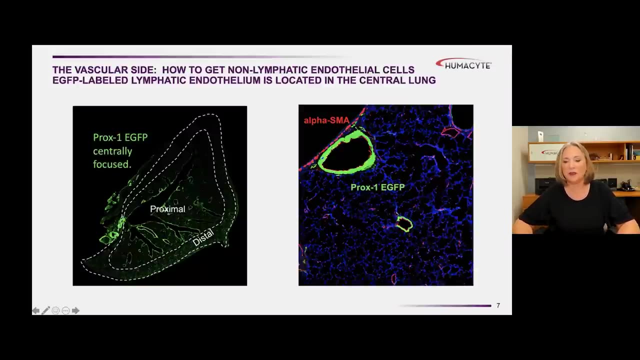 And these lymphatic endothelial cells express a transcription factor called PROX-1.. So, as you can see in this image, On the left, in the central portion of the lung, particularly lining the airways, is where the majority of the lymphatic endothelium resides. 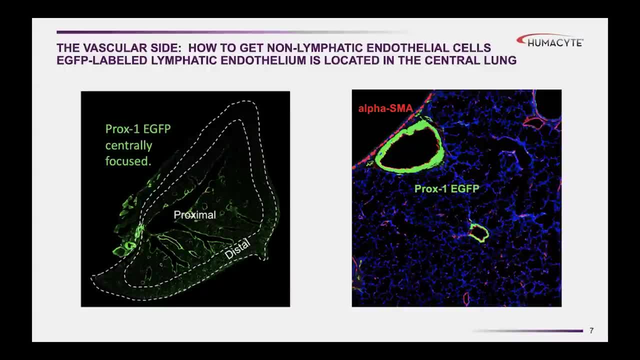 And that stains green. And so we were able to develop cell sorting methods whereby we could digest whole rat lungs from these PROX-1 GFP rats And really select out the endothelium that was negative for GFP, So that we were really getting a purified cell collection of blood endothelium. 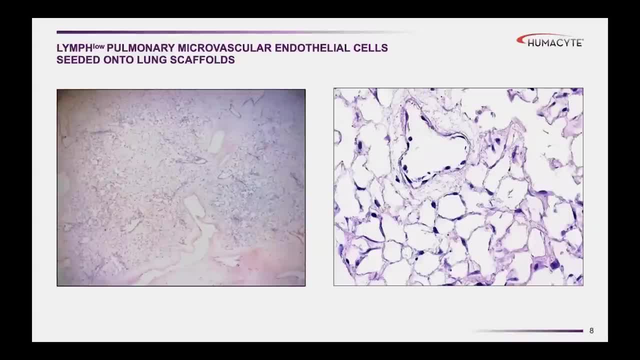 Which would presumably have higher barrier function. When we took these endothelial cells and seeded them into acellular lung scaffolds that we had decellularized in the rat- You can see it in a low power image on the left- That we were able to get fairly broad coverage of the microvasculature and the larger vessels in the lung. 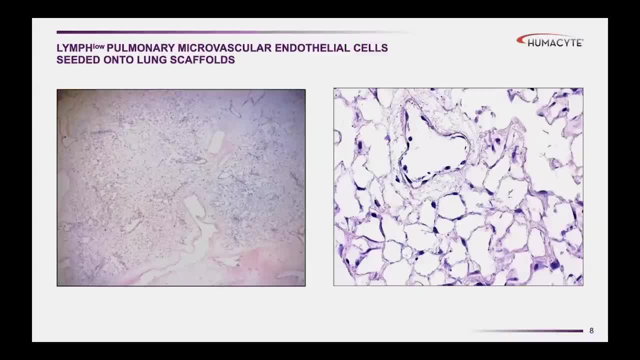 And you can see on the right. this is an example of blood endothelial Cell seeding into the acellular lung matrix And you can see that many of these cells permeate into the small microvasculature in the septae surrounding the alveoli. 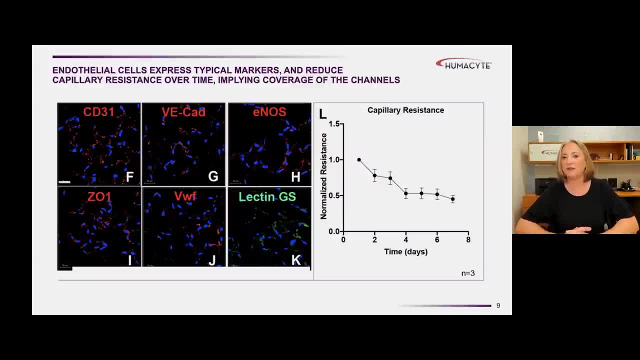 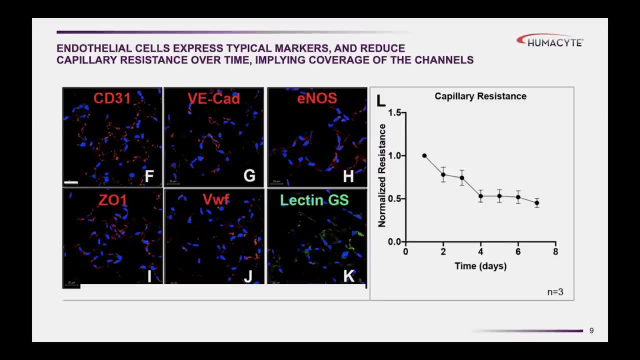 When we look at marker expression of these cells that are seeded into the lung, We can see that the blood endothelial cells express a lot of markers that we would expect to see in native microvascular endothelium, Including CD31, V-cadherin, endothelial microcarcinoma. 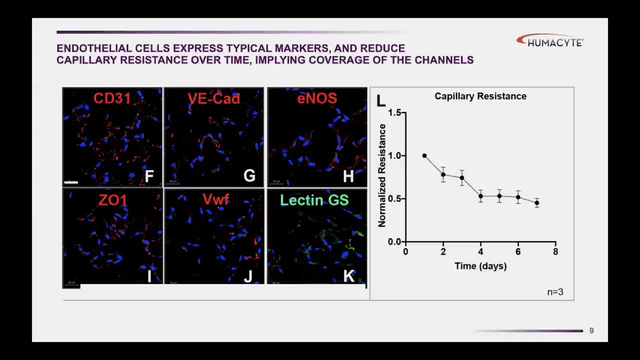 Endothelial nitric oxide synthase, VWF, and also Zona occludens. 1. Which is an important molecule for forming tight junctions and forming barrier in between endothelial cells And, as you can see from this image on the right, 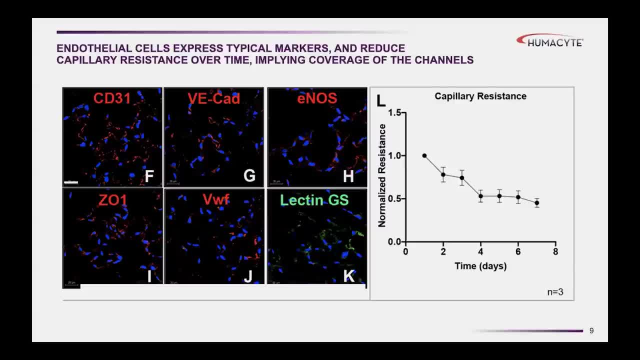 When we measure the resistance of the capillary bed, Which we're able to do by flowing culture medium through the vasculature And by measuring pressure drops across the vasculature over time And we can calculate a capillary resistance. What you can see is that over time, as the endothelial cells migrate into the microvasculature and begin to line the conduits, 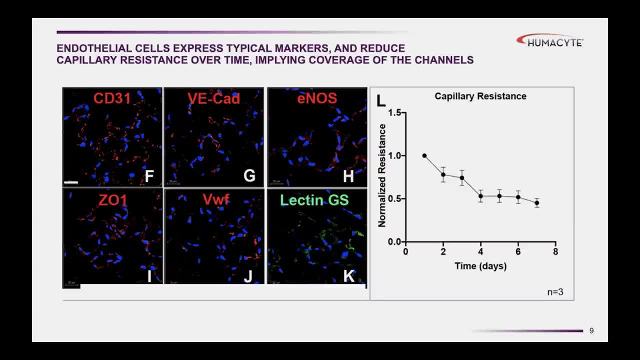 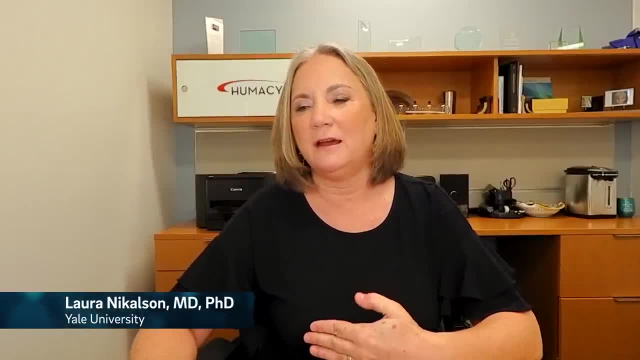 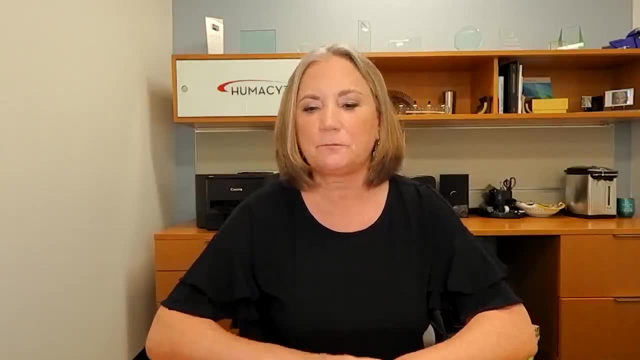 We see that the capillary resistance actually goes down over time, And we viewed these as sort of positive indicators that the endothelial cells were adhering to the walls of the vessels and doing what they were supposed to do. We then also performed assays. 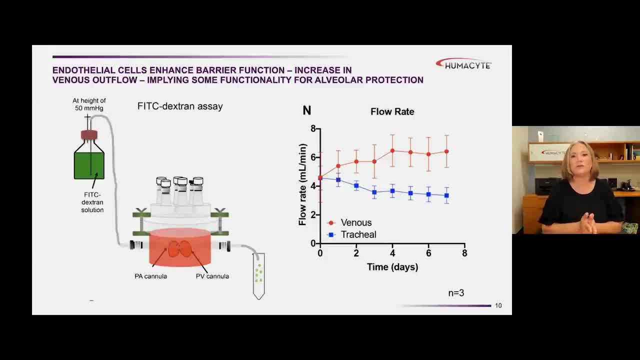 That measured not just the resistance of the vasculature But also the barrier function. So one of the key functions of the lung microvasculature and the epithelium Is that it forms a tight barrier between the air in the air sacs and the blood in the microvasculature of the lung. 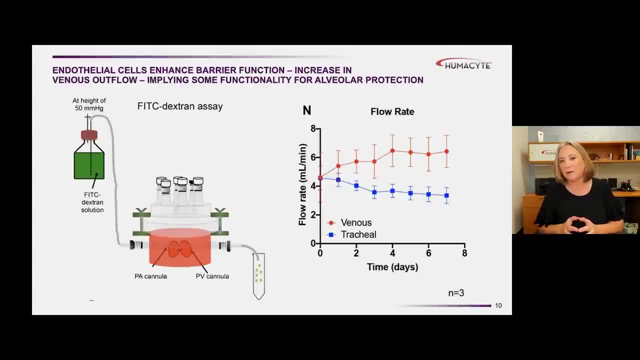 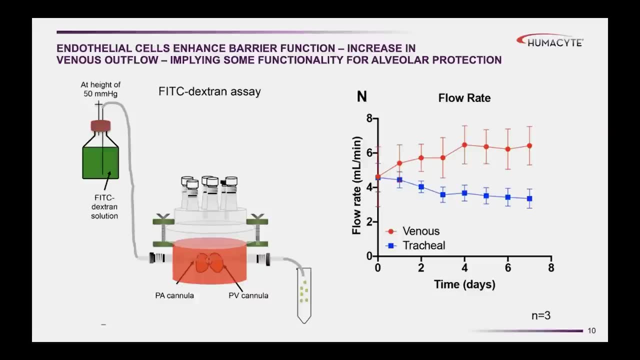 And so the ability to recapitulate that barrier function So that you don't get transudation of fluid Across the alveolar barrier is really a key aspect of whole lung engineering. And what we found when we measured a barrier function or essentially, flow rate, 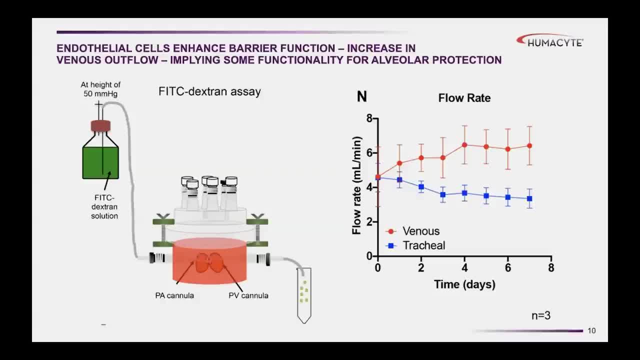 Liquid flow rate going across the alveolar barrier from the vascular compartment into the airway compartment. What we found is that flow across that barrier tended to go down over time as the endothelial cells were cultured in the vasculature, And you can see this image on the right. 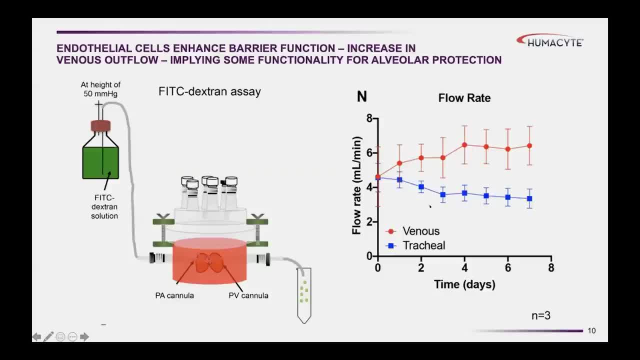 These, these, these blue squares show that there's a slight decrease in fluid flow across the barrier And, going along with that, that there's a concomitant increase in vascular flow, that that enters the pulmonary artery and then exits the pulmonary vein, And while these are both things that we would like to see, 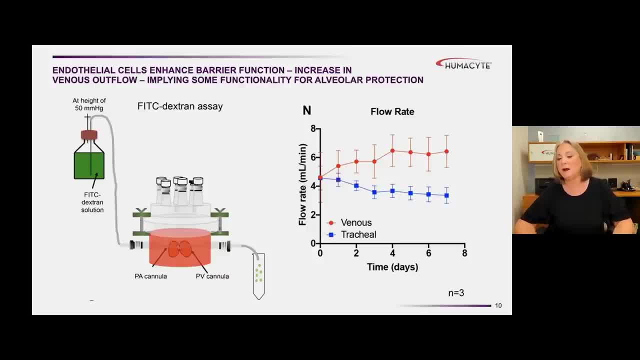 What's important to note is that the flow rate in blue boxes here certainly does not go to zero over time. So that means that there's still quite a bit of The fluid transudation from the, from the vasculature, into the airways. And- and that's a nice- that's a nice way of referring to drowning. actually. So if you, if you put a lung that's very leaky into an animal or into a human, then you'll get that fluid transudation into the airways and you'll basically drown the recipient. 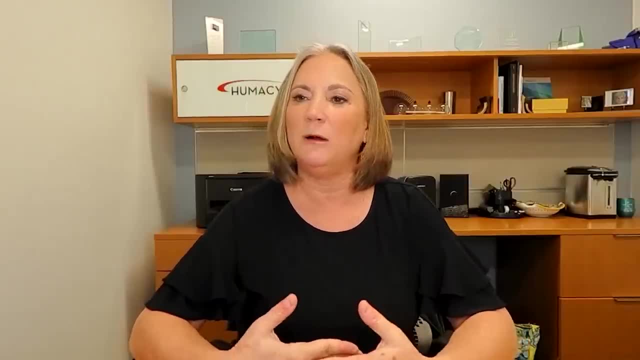 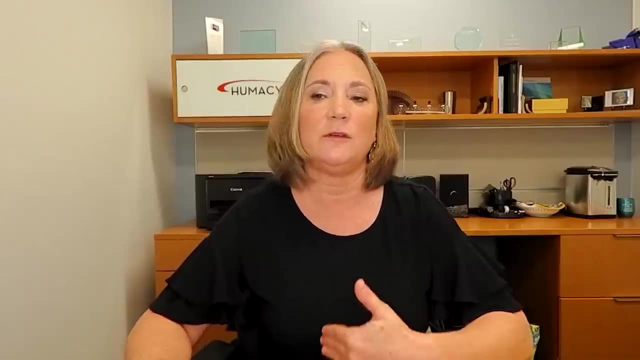 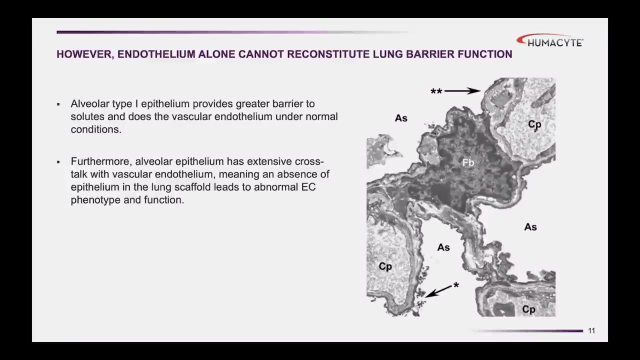 So? so the message here is that, while while providing blood endothelial cells into the microvasculature Certainly helped with decreasing resistance and increasing barrier, and while it was helpful in our hands, it was not sufficient. So, then, that that caused us to look a little bit more carefully at not just the endothelium on the vascular side, but also to try to understand how the endothelium interacts with other cell types. 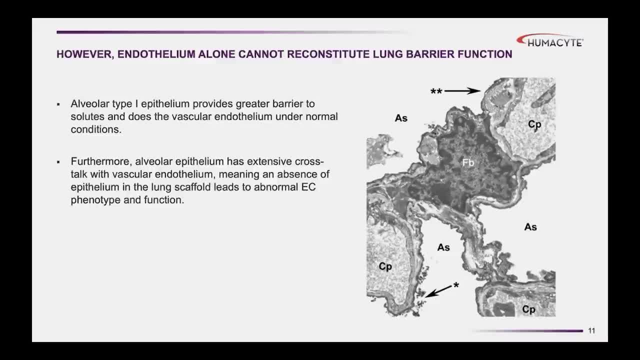 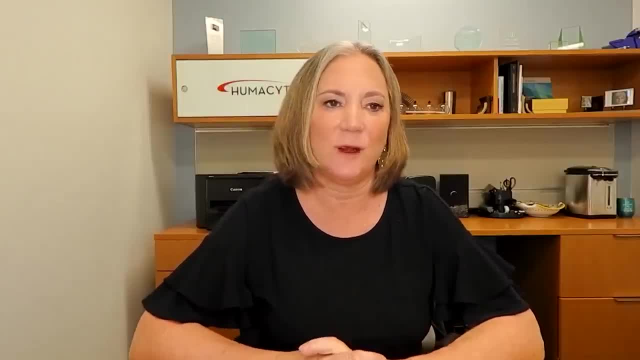 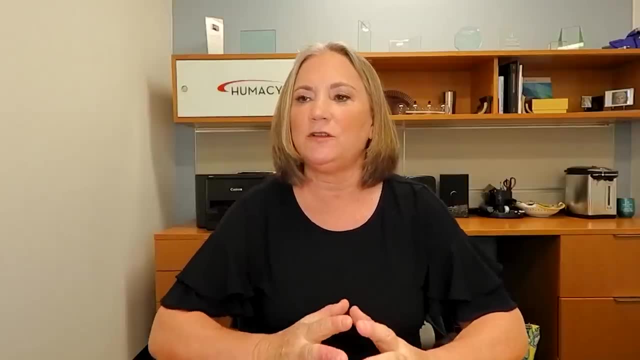 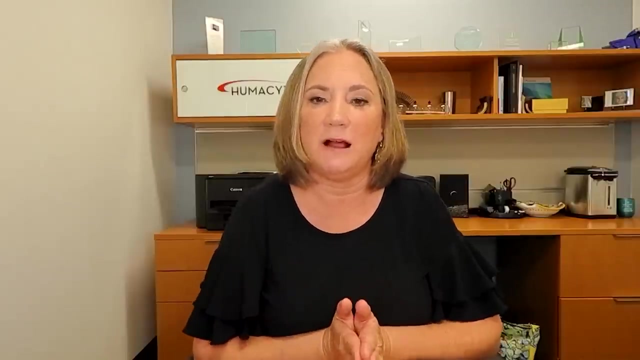 In in the alveolus to maintain homeostasis and also to try to maintain barrier function, And this led to a set of experiments that was done By a very talented graduate student in my group group group named Katie Leiby. She's an MD PhD student and what she, what she wanted to understand was the impact of different cell types, particularly endothelial cells, but also alveolar fibroblasts. 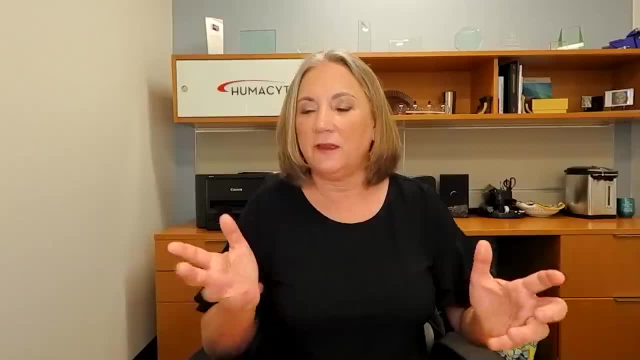 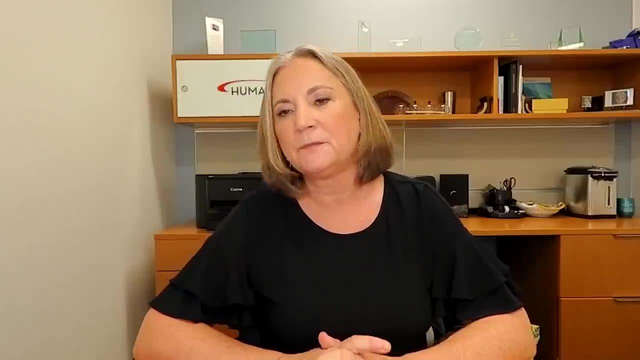 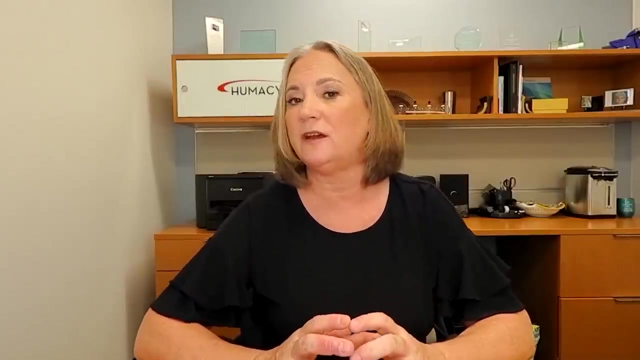 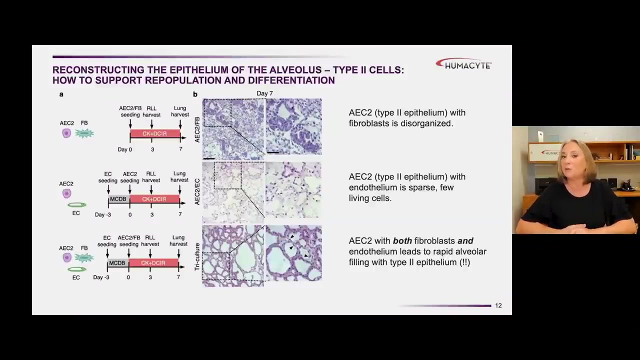 On the differentiation and the growth of the, the, the epithelial stem cell of the lung, which is really the type two alveolar epithelial cell. So so in our Alveoli that there are really two flavors of of epithelium: there at the type two cells which makes surfactant and which allow our lungs to expand, but they're also the local progenitor cell for the type one epithelium. 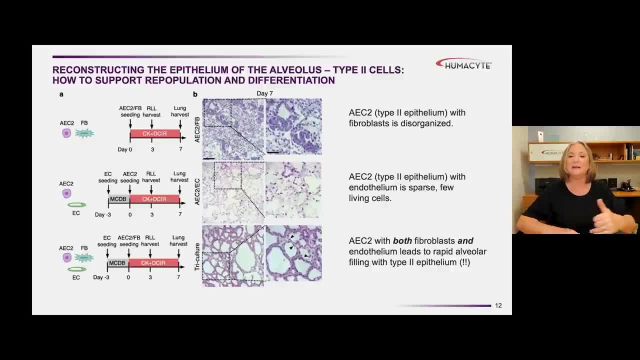 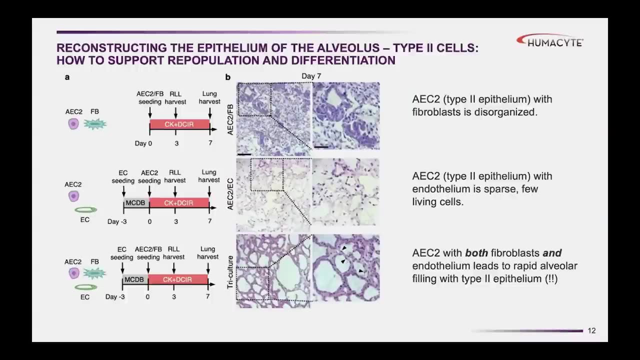 And the type one epithelial cells are the cells that really line most of the surface area of the alveoli and provide a lot, of, a lot of barrier function. And so what Katie found is that by by combining A really type two epithelial cell conducive medium, combining that with co culture with both epithelium fibroblasts and endothelial cells, 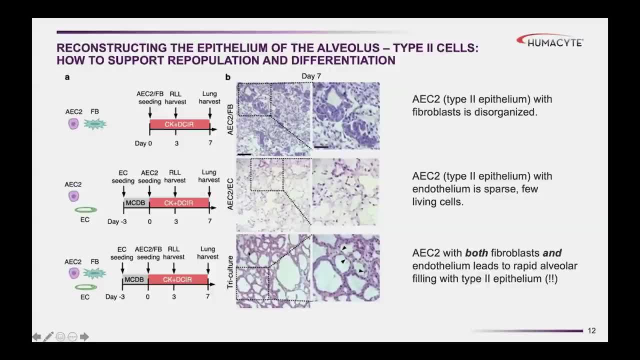 She found that she was able to form really dense rings of alveoli that were lined almost entirely with type two epithelium, Which is actually kind of an extraordinary finding, Because it means that she was able to essentially reconstitate the epithelium. 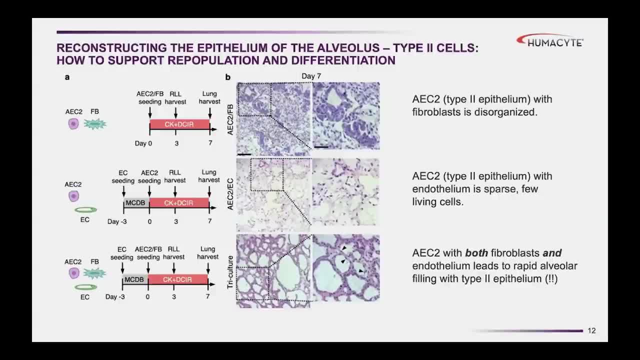 The epithelial component, you know, across an entire organ in a fairly organized fashion. what she also found was that when she just seeded the, the, the epithelial progenitor cells, just with endothelium, that that that the growth of the of the epithelium was poor, and if she seeded them with just fibroblasts, that there was a lot of epithelial cell growth, but it was very disorganized. 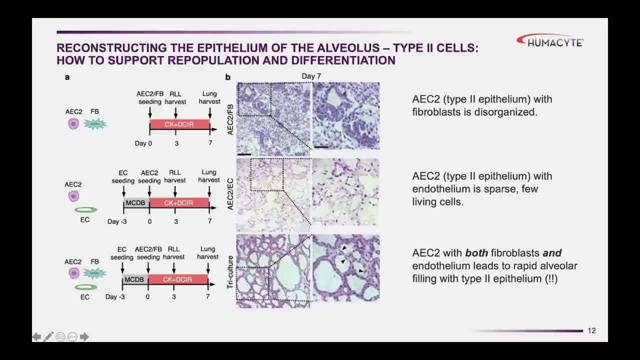 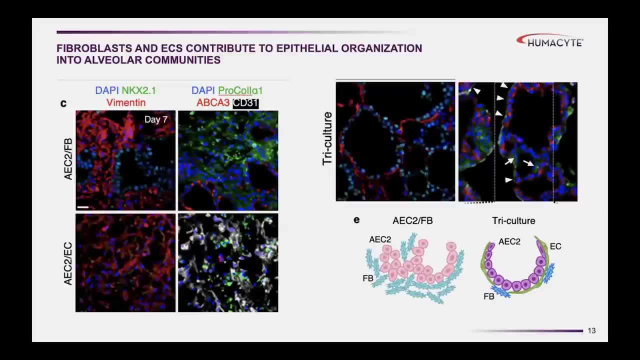 So having these two other cell types was really pivotal for for generating alveoli. So we have a button, A local study in the lab that showed that there were six or seven cells that were associated with alveoli. This is their number one: alveoli. 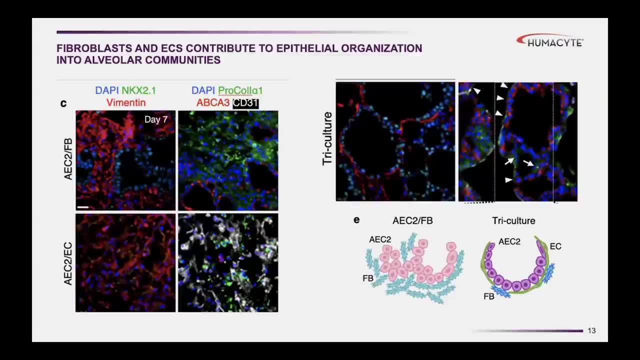 So if you had a culture with an alveoli cell, an alveoli cell follows by a macular cell And they're now a molecular structures that contain really robust epithelium. And if we look at this a little bit more closely, 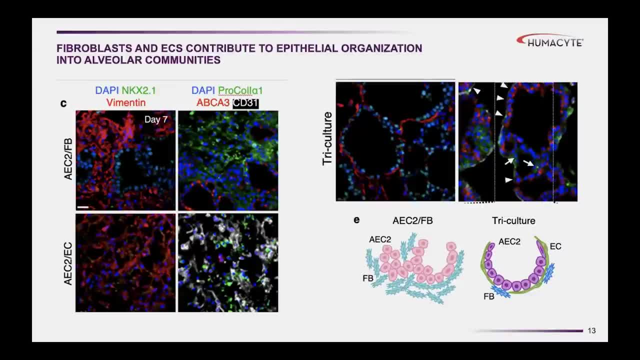 Again there's. there's some, you know, standing here for some markers that may not be familiar to some folks if you don't think about one all the time, But But essentially what what this staining shows is, that is that in Tri culture lungs. 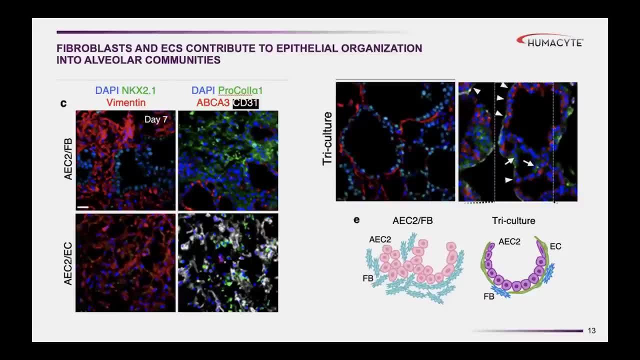 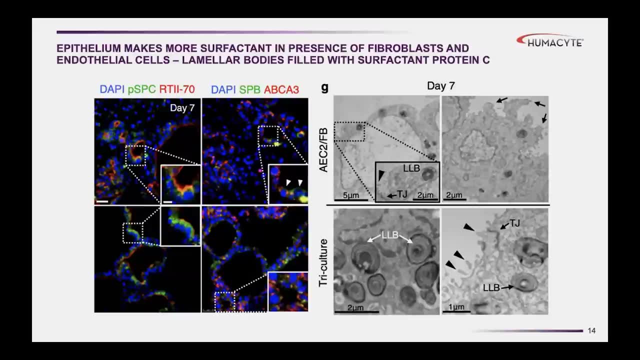 We got a tremendous amount of markers, which is ABCA3, and also vimentin and NKX2.1.. This just shows even a little bit more detail looking at the functionality or the ability of these type 2 cells to make an important 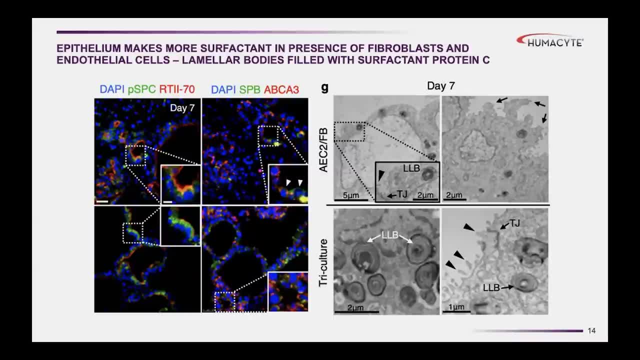 molecule which is surfactant molecule, which allows our lungs to inflate and lowers the surface tension in our lungs. Surfactant molecules are stored in lamellar bodies and you can see that in triculture the type 2 cells have huge numbers of lamellar bodies which contain 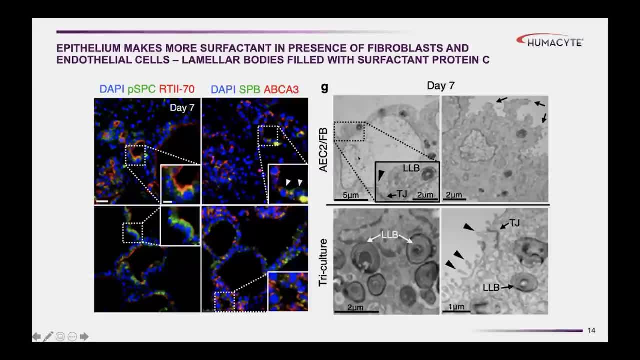 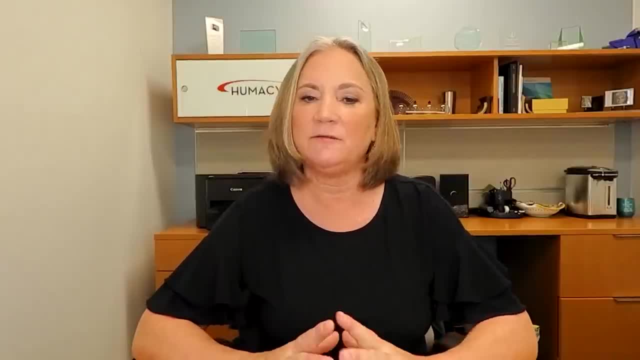 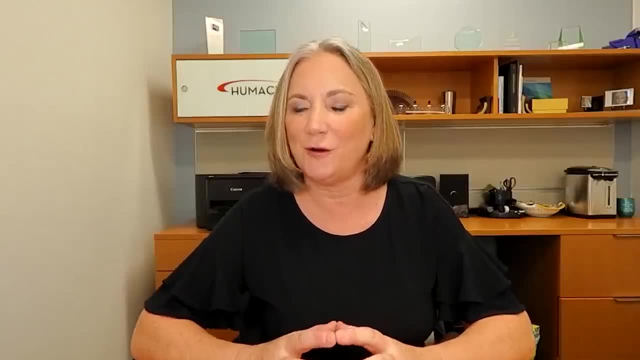 surfactant that's waiting to be released from the cells. When we don't have triculture, we see many fewer of these lamellar bodies. To finish up, I'm going to focus a little bit on some of our single cell work that has really tried to understand. what are the conversations that are? 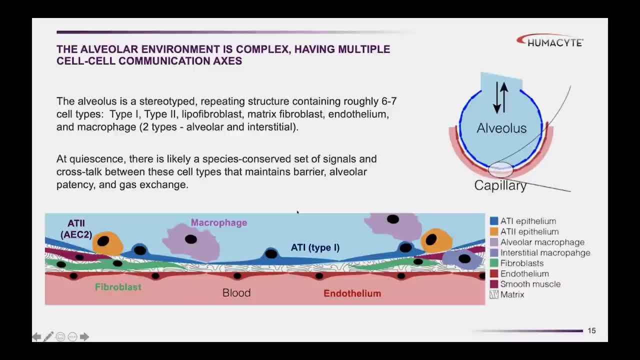 going on between the different cells in the alveolus. This is really a cartoon of these type 2 cells. This is a cartoon of these type 2 cells. This is a cartoon of these type 2 cells, different cell types that we think are important and are present. As I mentioned, there's the type 1. 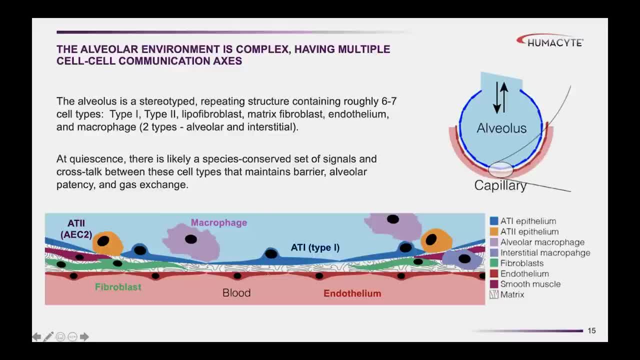 epithelial cell which covers most of the alveolus. There's the endothelium, the blood endothelium, which sits on the other side of the basement membrane. Those two cell types, which cover most of the surface area, are really separated by only about 50 or 100 nanometers. It would not be. 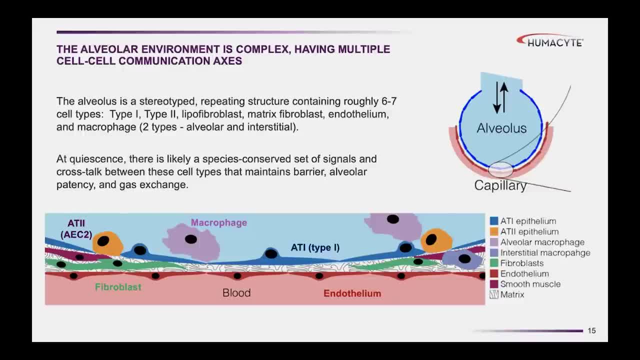 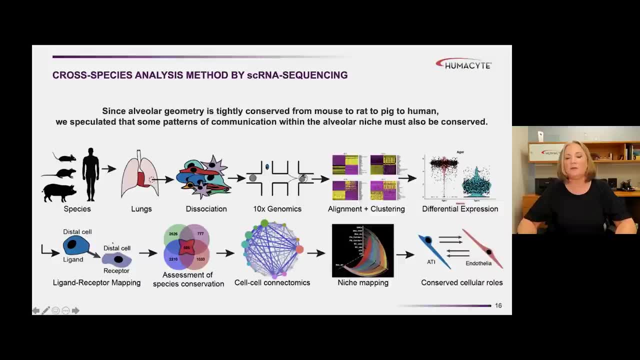 surprising if those two cell types actually had very active conversations with each other. In addition, there's type 2 cells, there's macrophages and there's a couple different flavors of fibroblasts. In order to understand in a very broad way how cells in the alveolus talk to each 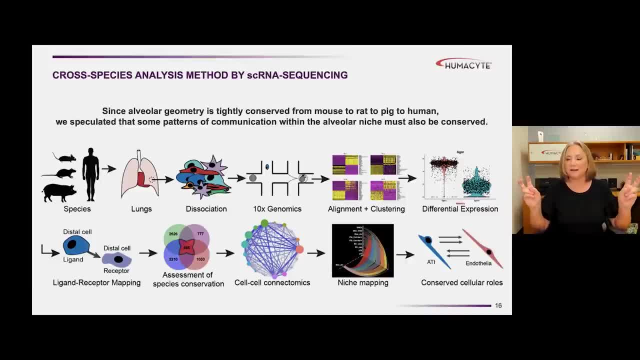 other. we really wanted to get a signature of longness, a signature of what the alveolar communication system looks like. To do that, what we did is a single cell analysis of the connectomics between cells in the alveolus, but not just in one species. 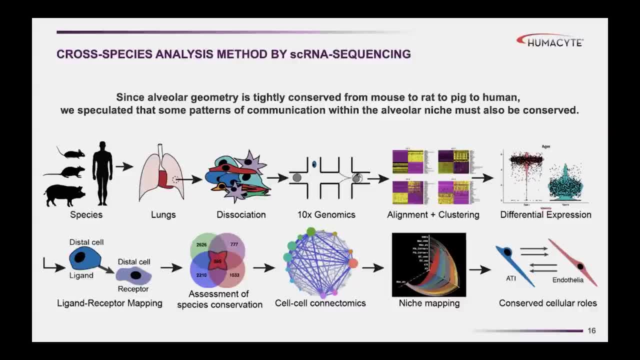 We actually looked in four species. We looked in mouse, rat, pig and human. Our goal was to not have species-specific communication algorithms that we were focused on, but really to try to understand what is it about this collection of six different cell types that creates homeostasis? 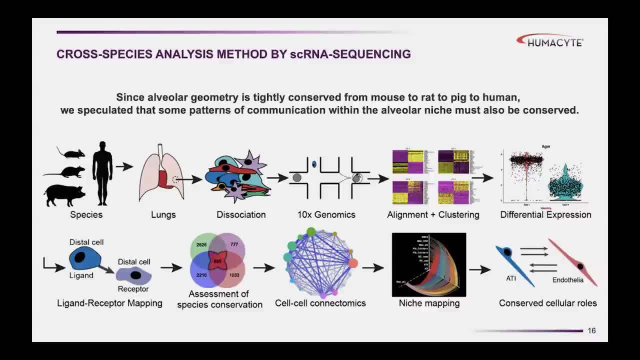 across alveoli, across all of these species. A rat alveolus looks a lot like a human alveolus. We speculated that the alveoli above the mouse would have similar signaling. This is just one example of one signaling vector that we identified. that's certainly not surprising. 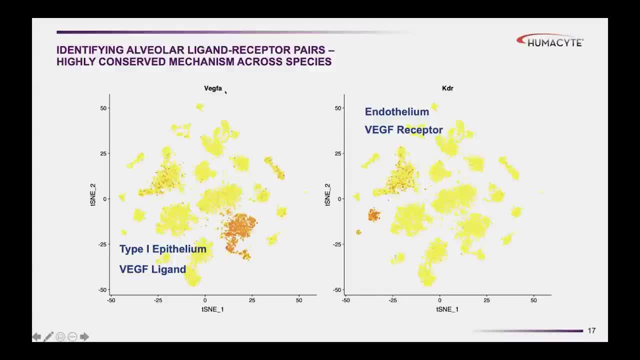 This is some single cell data. looking at the expression of VEGF-alpha, As you can see, most of the VEGF is actually made by this cell cluster here, which is actually the type 1 epithelial cells in the alveoli. Similarly, if you look for the receptor for VEGF, you see that it's. 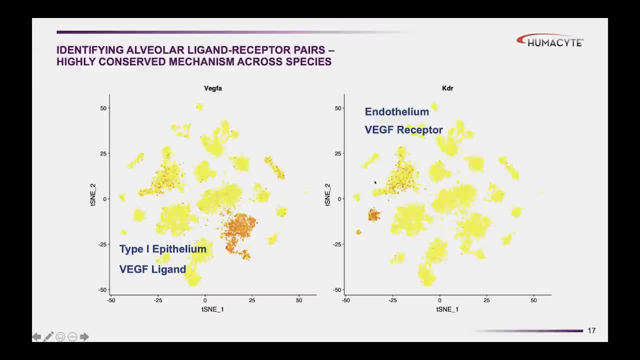 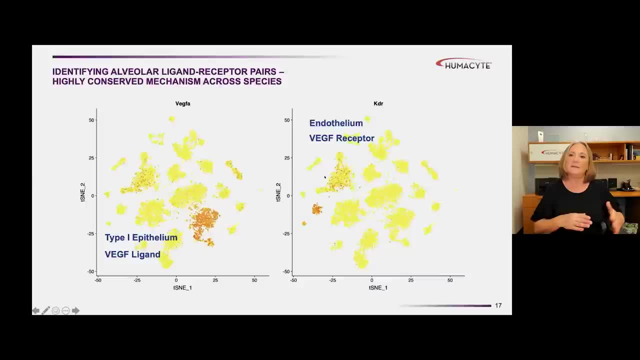 that it's located almost entirely on the vascular endothelium, as you would expect, And so by by looking at these two sets of data, we can essentially draw a vector- that for a signaling vector- that connects the type one epithelium to the endothelium in the alveolus.